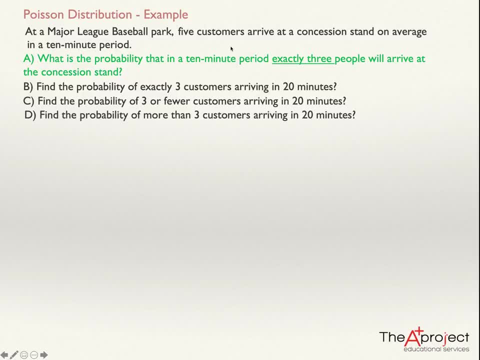 And second this function. this problem tells me actually the average of these numbers. So we know the average of this random variable in a period of time. So if we know that, if we know that this is a discrete random variable and at the same, 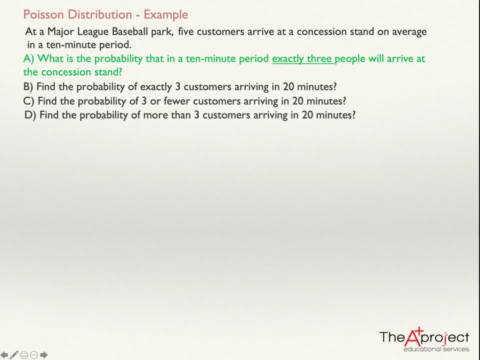 time. we know the average in a period or interval, we are thinking that would be a good idea to use the Poisson distribution. So let's get a solution of this problem. So because I noted that this is a Poisson distribution problem, I'm going to type here: 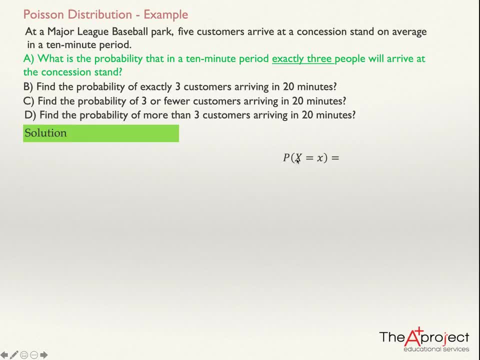 the Poisson distribution formula. So the probability that the random variable x takes the value x will be equal- I can't write this Or I can't write this, Or I can write the probability of x, the value x. it will be equal to e, to the power. 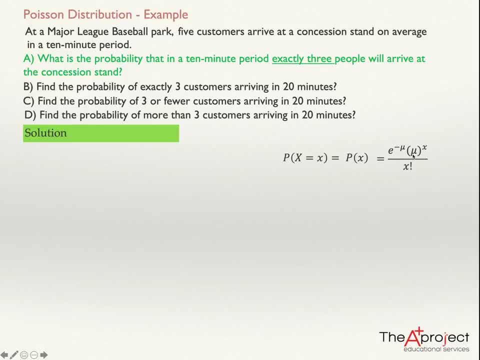 the mean negative times, the mean to the power, x divided by x factorial. So and what information I have in the problem? I know this average five customers arriving per 10 minute period. So lambda will be equal five. But this is not necessarily the mean that I need to put into this formula. 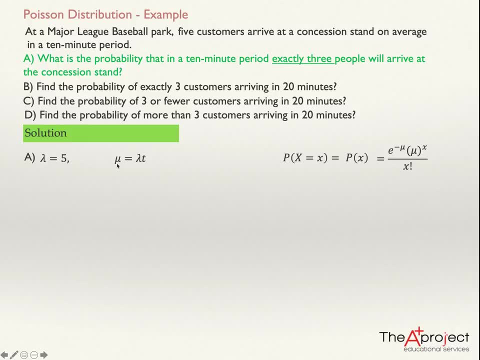 So the mean that I need to put in this formula will be mu equal. this lambda times t, And t will be the number of the periods, the information periods and the information periods are 10 minutes. 10 minute periods. That appears in the questions periods. 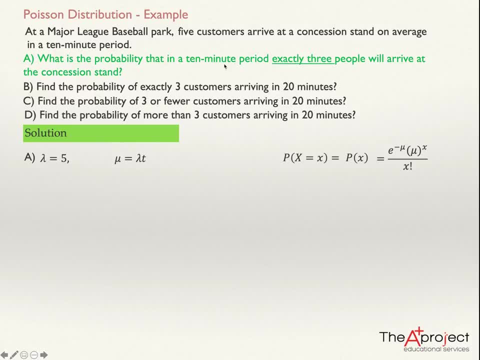 And the periods in the questions are again 10 minute periods, So there is only one. it's the same 10 minute period in the information in the question, So t equal one. This is, for example, in the second question, 20 minute period. 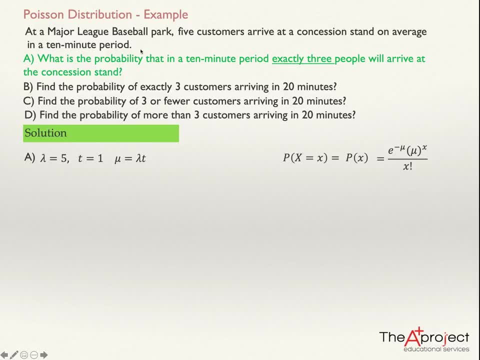 And the information was in 10 minute periods. I noticed that t equal two. Then this: for answering the question b, I will be using t equal two, But in this case it's the same: 10 minute and 10 minutes. 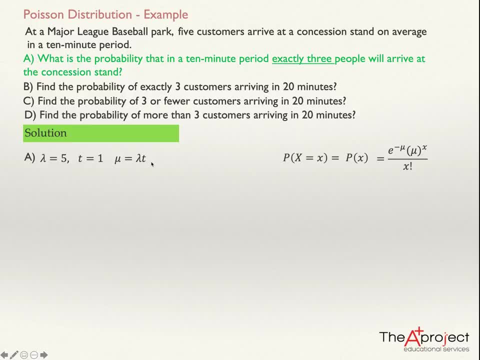 So mu and lambda are the same number. So mu, this will be five times one, equal five. So I can put this five into the formula. So the mean is five And, depending on the question, I will be using the x, Because the question is: 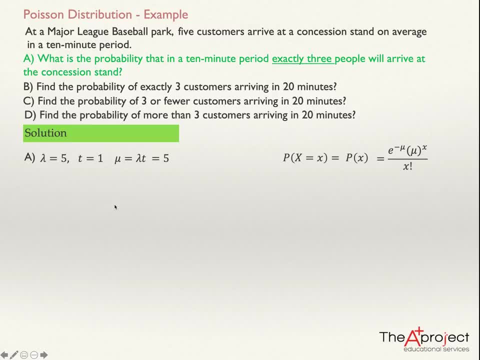 What is the probability of exactly three? So it will be p of three. So x equal three And the probability of x equal three. I can write in this way or I can type in this way: probability of three. So it will be e to the power negative mu, but mu is five to the power negative five. 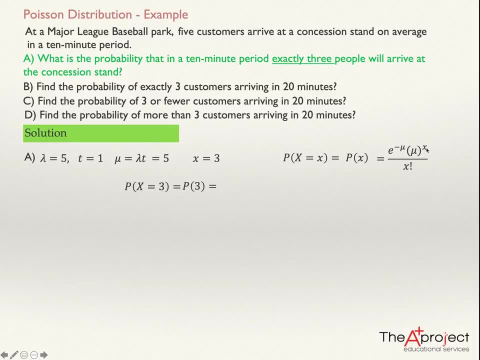 times five to the power three, Because the question is now probability of three. So mu is five, So x equal three And divided by three factorial. So let's type this: e to the power negative five, five to the power three divided by three factorial. 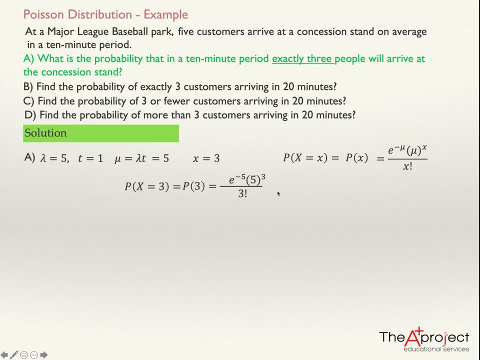 And then you can use a calculator to compute this And the answer will be 0.1404.. Good, So you can do this for solving a problem like this. You can solve a problem like this also using Excel. So what to do in Excel? 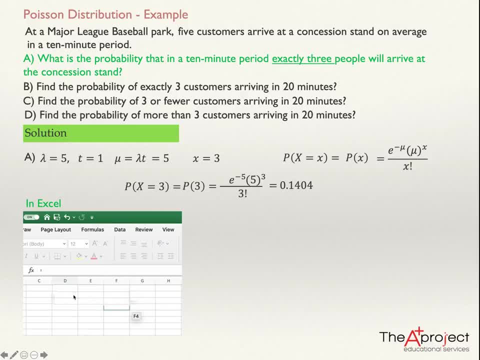 So open Excel And if you have Excel, in whatever cell of Excel's worksheet you can use, you can type the function for the binomial- sorry, the Poisson distribution, And this is Poisson distribution. So you write Poisson dot distribution. 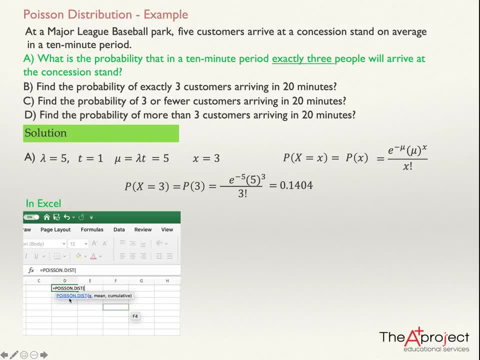 And if you do that, immediately Excel asks you for what to type. So you need to type the value of x, And you know the value of x is three. You need to type the mean after a comma, And the mean is five. 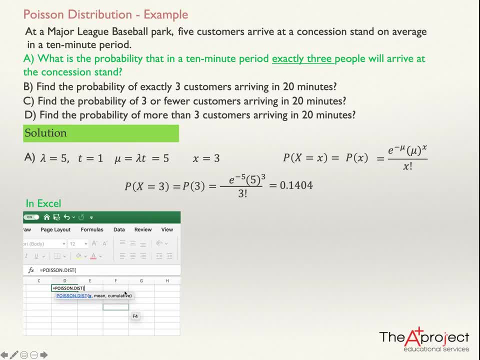 And then you need to tell Excel if this is a cumulative problem or not. It's not a cumulative problem if the question is exactly Exactly. So for this problem you need to answer here that this is not cumulative. So you can type false or you can type number zero. 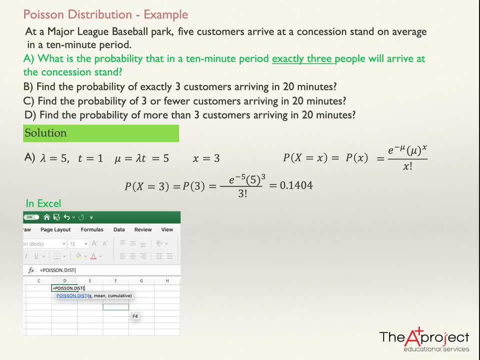 Number zero means the same of false. in Excel, Zero is shorter, So for that reason I will be typing zero. OK, So you need to know what to type. You see this? That's why you need to type Equal Poisson distribution. 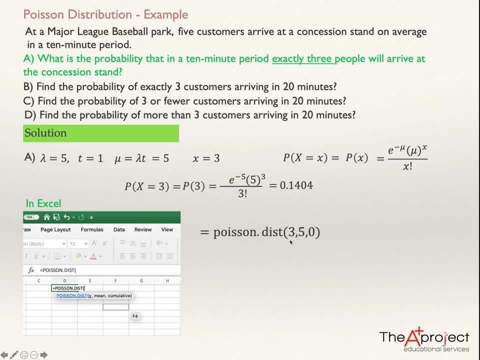 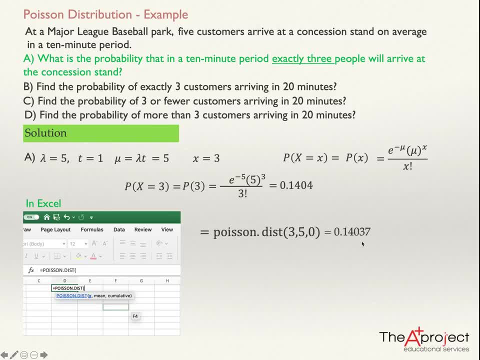 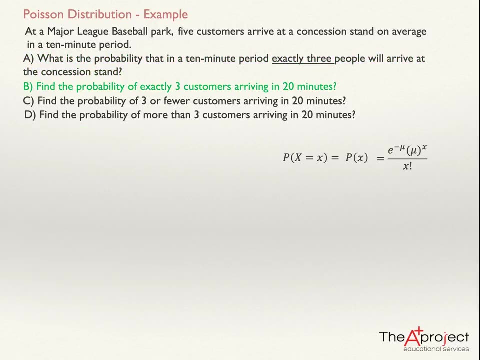 will be the same as before. yeah, Obviously, here the Excel is telling me the answer. we try in decimals, or sometimes they give you the answer with more decimals, And that answers the first question. And now all you apply on point B. So let's go now to study the second question. 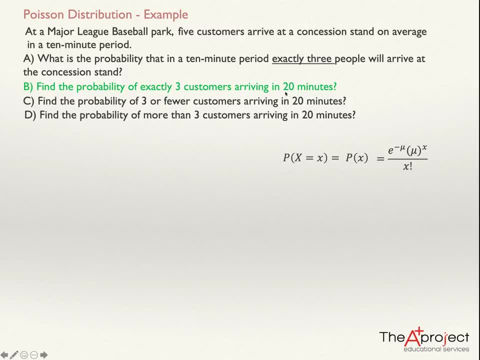 Find the probability of exactly three customers arriving in 20 minutes. So if this is the case in 20 minutes, the value of x continues being 3, but now the value of mu, maybe, will be different. So the information I have here will be b for the question. b will be that lambda equals. 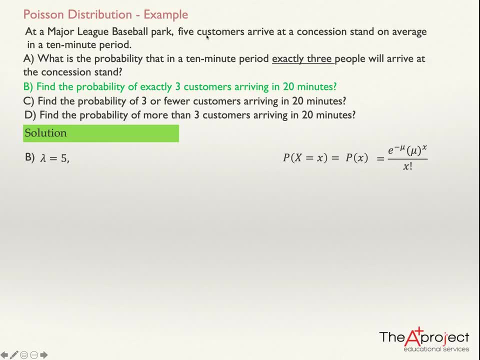 5. This is the mean in the information, and the information of the problem told me that five customers arrive on average in a 10-minute period. We need to type here, not this lambda. we need to type is mu, but mu is lambda t. 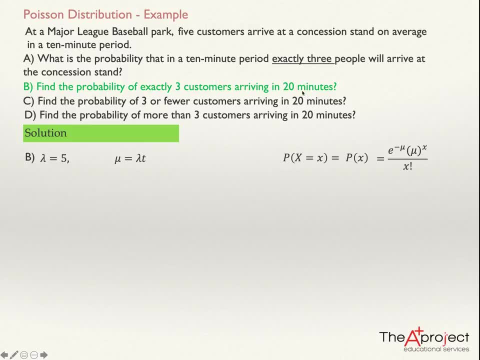 T is the number of periods in the questions. How many periods? How many periods in the questions related to the periods in the information of the question. So this is a 10-minute period, this is a 20-minute period. There are two of these periods here. yeah. 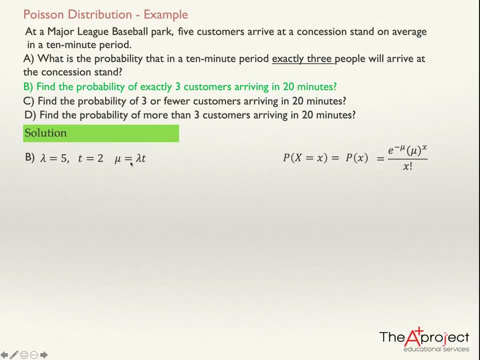 So for that reason, t equals 2.. So to know, mu will be lambda 5 times t times 2, so mu equals 10.. Mu equals 10.. Now we have the value of mu to put into the formula. yes. 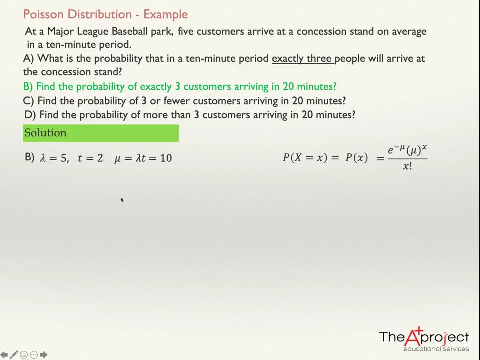 So because I have the value of mu, now I can type: so x equals 3, so the probability of the random variable takes the value of 3.. That is the same writing probability of 3, but in this case what we are going to use. 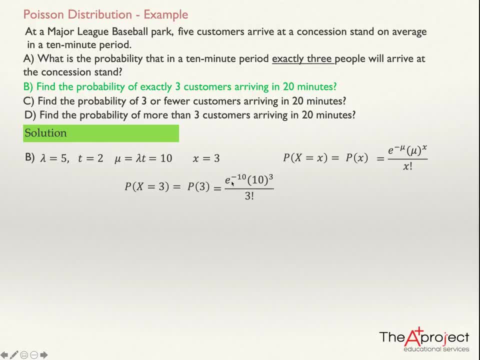 is mu equals 10.. So it will be equal e to the power negative 10,, 10 to the power 3, over 3 factorial. OK, OK. So please use a calculator to find this question, to find this answer. 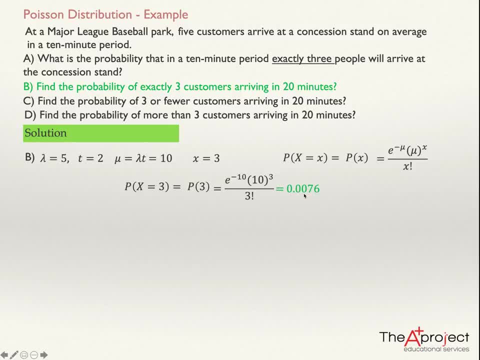 So the answer will be 0.0076.. If you are going to solve a problem like this in Excel, then open Excel and in whatever cell of the world should just type Poisson. Don't forget to type the equals signs first. 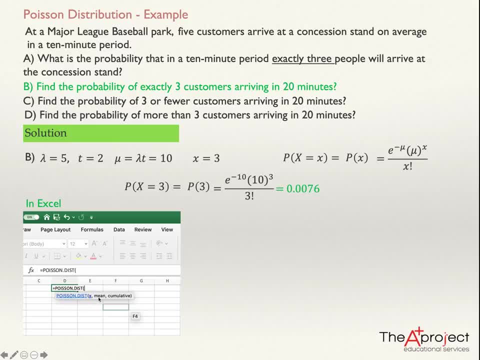 So the value of x is 3.. The value of the mean is 10 in this case, and this is not cumulative. yeah, The question is exactly 3.. So, for that reason, what you need to type is this: equal Poisson distribution 3, 10,. 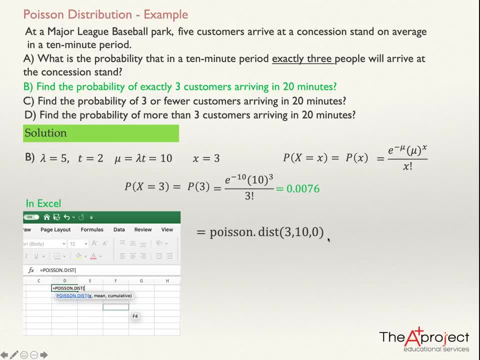 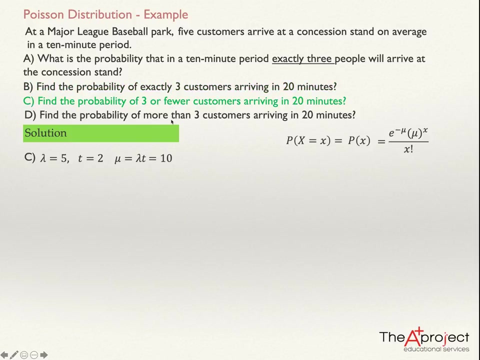 0.. If you press Enter now after you type this, you get the answer 0.00756667, round your answer as needed. OK, OK, So this will be the answer of question B. How to answer question C. 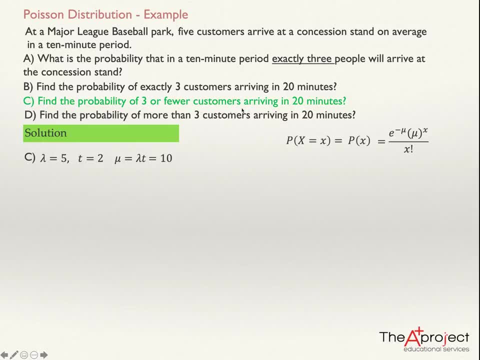 So find the probability of 3 or fewer customers arriving in 20 minutes. So this is the question. So what I ask you Is: with a probability that the variable take the value 3 or less than 3.. So the probability that the variable x will be smaller or equal than 3, less or equal, 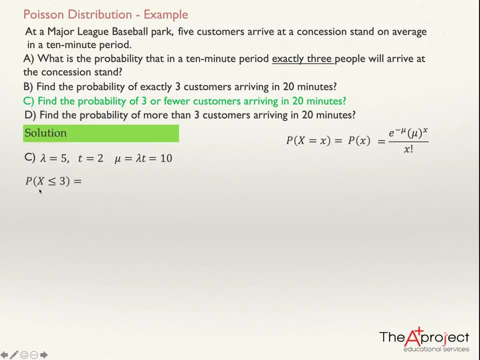 than 3.. And how can be a variable x be less or equal than 3?? Maybe if it's 0, or 1, or 2, or 3.. So this probability, The probability will be the probability of 0, plus the probability of 1, plus the probability. 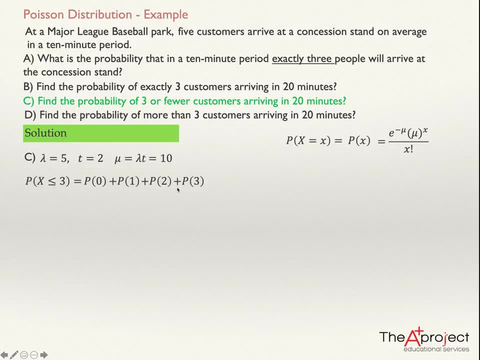 of 2, plus the probability of 3.. So what you need to do is compute each of these probabilities and add together. Let's do that. The probability of 0 will be equal e to the power negative 10, remember mu equal 10 in. 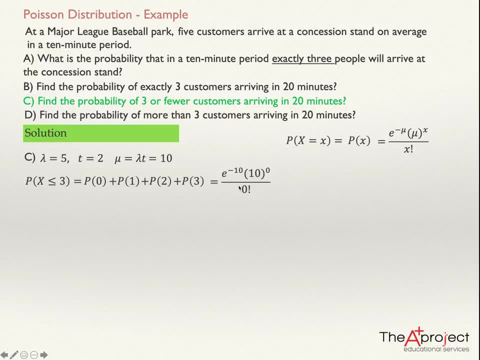 this case We have 20 minute period. So 10 to the power 0, divided by 0 factorial Plus. now do the same: The mu continue being 10.. But now x will be equal 1.. Plus, just make a substitution of x instead of typing x type 1.. 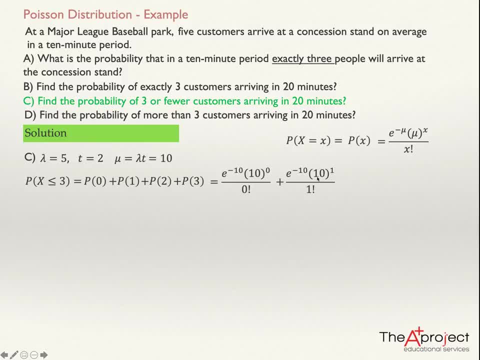 And the value of the mean continue being the same. Yeah, So plus again, the same. the same for the value of the mean, but now the value of x is 2.. And this is the probability of 2, plus the probability of 3.. 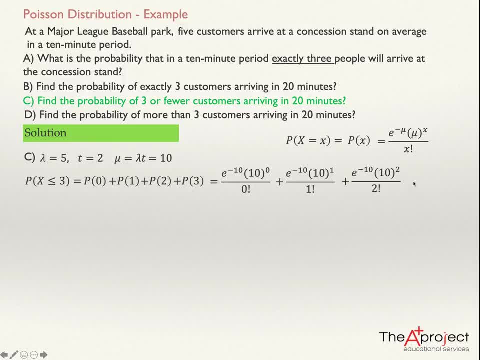 The probability of 3 is the one that we computed before. Yeah, But this is, remember, e to the power negative 10, plus 10 to the power, 3, divided by 3, factorial. So you can solve each of these and add together and you get the answer. 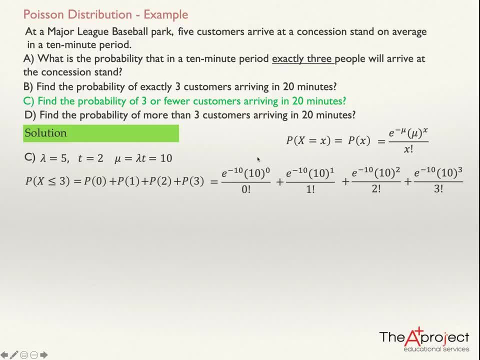 An easiest way to work will be if you noted that the e to the power negative 10 is a common factor, So you can actually put e to the power negative 10 as a common factor. open bracket and put into the bracket what remains after you take it out. this e to the power negative 10.. 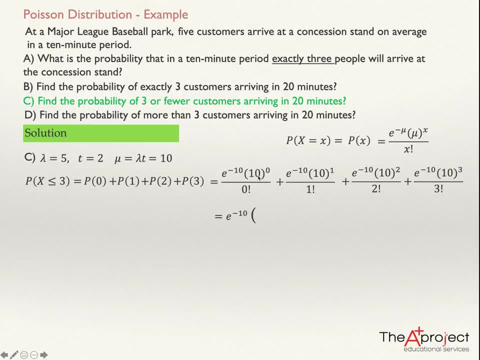 So, for example, here is 10 to the power 0, divided by 0 factorial. By the way, 10 to the power 0 is 1.. So it will be 1 over 0 factorial. 0 factorial is also 1.. 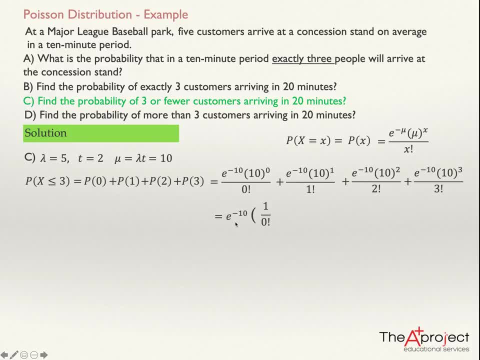 Here, for example, e to the power negative 10 is already written outside of the bracket, So it will be plus 10 to the power 1, that is this thing divided by 1 factorial. 1 factorial is also 1.. 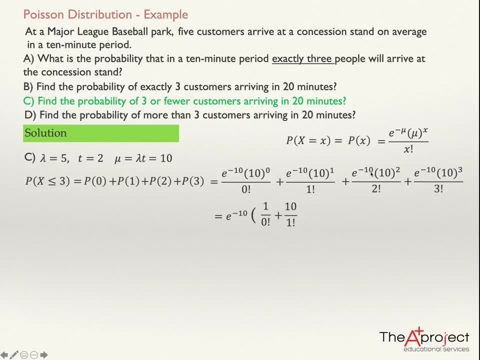 You can type here: 1. Plus- this is already written outside of the bracket- Then 10 to the power 2.. 1 factorial- This is 100, divided by 2 factorial. I'm going to type 10 to the power 2, divided by 2 factorial. 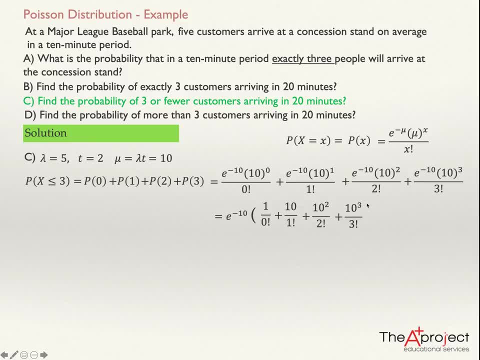 Plus 10 to the power 3, divided by 3: factorial. Close the bracket Then after. if you do that, maybe you can find the answer easier. So this is will be 1 plus 10.. 10, 10 squares is 100 over 2.. 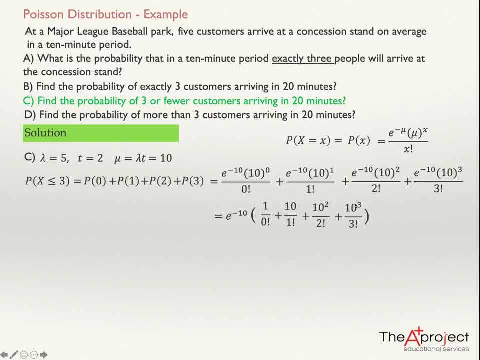 This is 50.. 3 factorial is 6.. This is 1000 divided by 10.. divided by six. but you can type all of this in the calculator and you can get the answer. the answer is zero point zero one, zero three. but one thing that is. 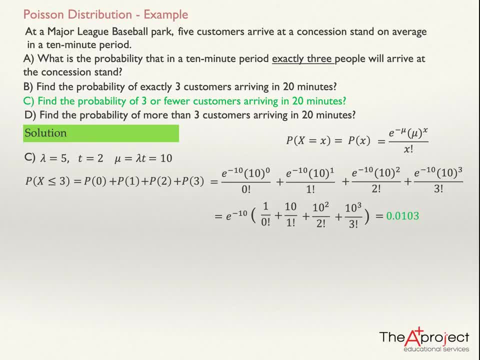 important. this was a cumulative problem. so the previous problems was where as getting the exactly three customers, but this is three or fewer, so less or equal than three. if we the question is like this, less or equal, we have accumulated problem and this is a cumulative distribution. then if you are 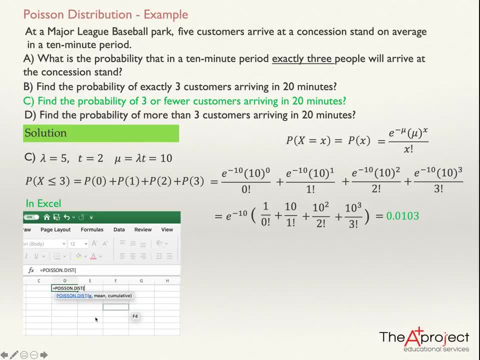 using Excel. you are going to do the same. you are going to type Poisson distribution, but instead of write zero for cumulative, you type one. so if you, if you want to know what to note, what to type is, this is what you need to type in a, in whatever cell of Excel: Poisson. 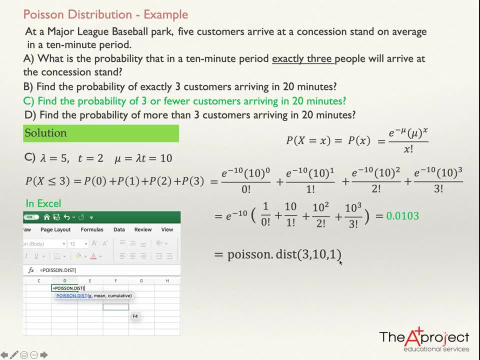 distribution: three ten one. if you do that, Excel give you the answer immediately after, after you enter. this will be zero point zero ten, zero three three six, and that give you the solution in the easy way, in an easier way, okay. so let's go to the, to the last question. find the probability of more than three. 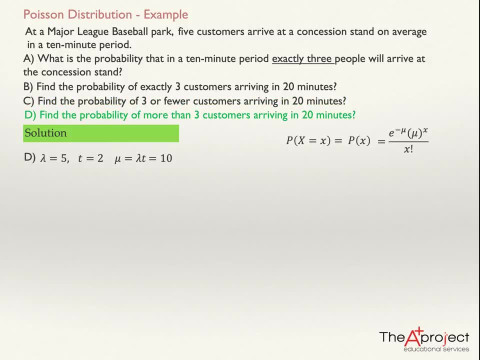 customers arriving in it in 20 minutes. so if that is the case, will be where we have. the same information is in 20 minutes. so mu continue being ten, but now. Now the question is probability of x greater than 3.. If the probability is x greater than 3,, 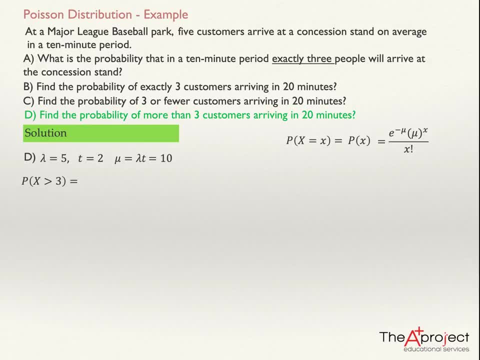 then probability of x greater than 3 will be 4,, 5,, 6,, 7,, et cetera. So it will be probability of 4 plus probability of 5 plus probability of 6, and so on. So you are never going to stop because it. 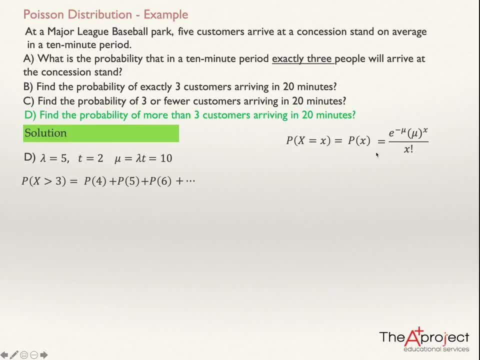 will be probability of 7.. So this will be: if you try to use the formula doing this, you're never going to finish, Or you will need to type an approximation, So this is a never-ending work. if you do that, The best way to do that is just to recognize. 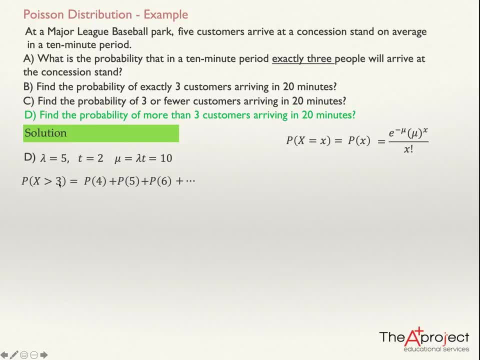 that being greater than 3.. And the probability of being greater than 3 is the same of the probability of being greater than 3, is the same of 1, minus the probability of x less or equal than 3.. Remember that adding together all the probabilities, 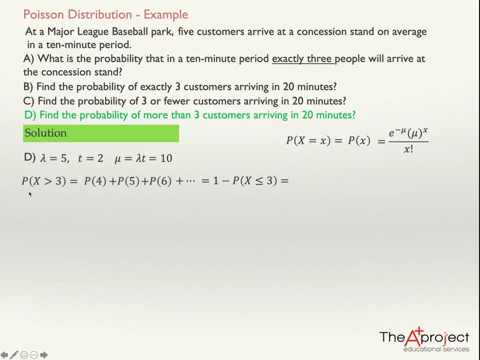 the answer is 1.. 1 minus the probabilities that are not here, that are, probability of 0,, probability of 1,, probability of 2, and probability of 3, will give you this. This: This is the answer for this problem. 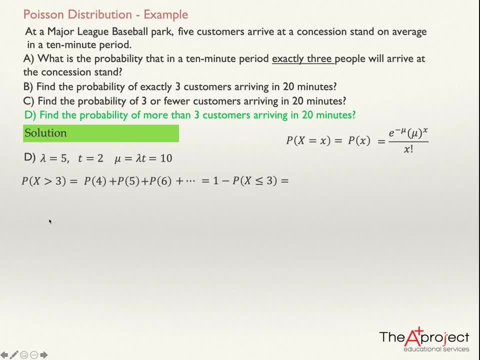 So if the question is probability of x greater than you can use, you can type 1 minus a cumulative probability. So, and the value of the cumulative probability will be the previous of the first one here. Here is 4, OK, previous to this 4.. 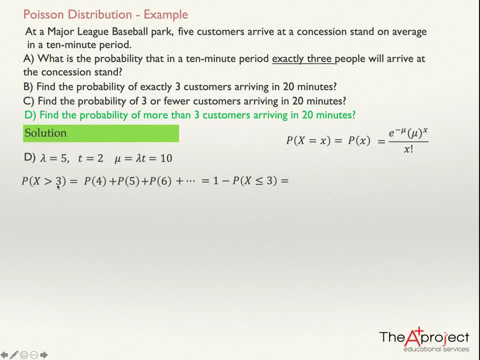 Oh, it's actually the same number that we computed before, So it's 1 minus 0.0103.. OK, So that will be the number that we computed before. So this is already known before. So it will be 1 minus the number that we computed before.